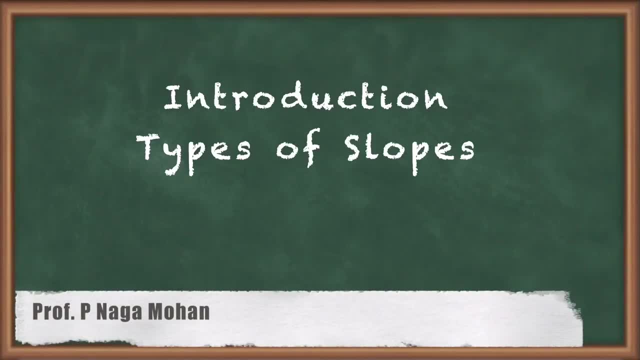 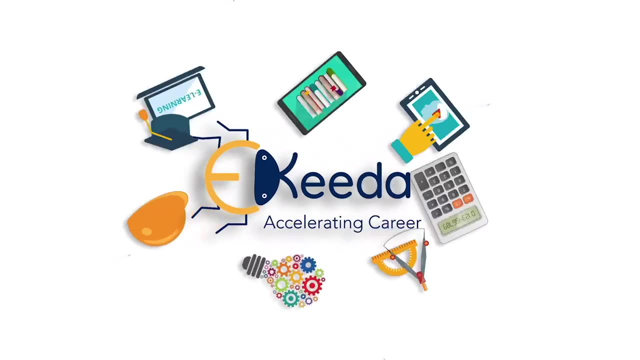 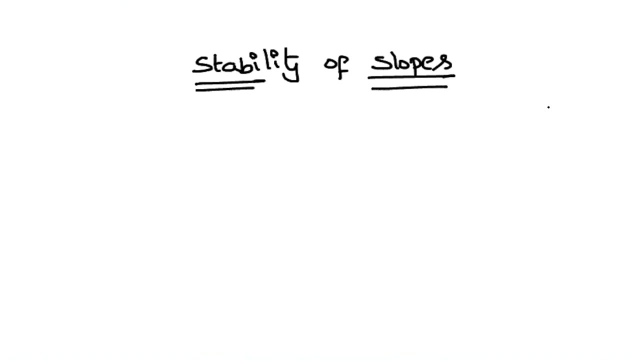 Hello friends. so here we are going to start a new chapter called the stability of slopes. So from gate exam point of view, from this topic we may get the two marks question. So instead of simply by hiding the formulas, if we can understand them, then definitely. 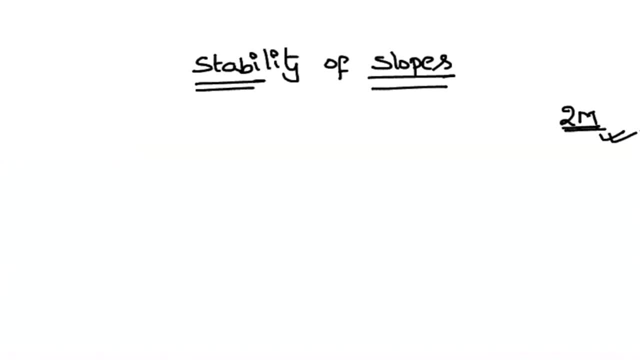 we can score easily these two marks without much difficulty. So the contents of this chapter will be: first we are going to study about the types of slopes, And then we will study about the types of failures, And then we are going to see the methods, different methods. 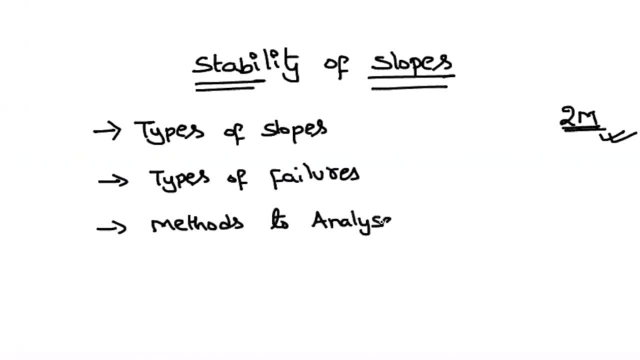 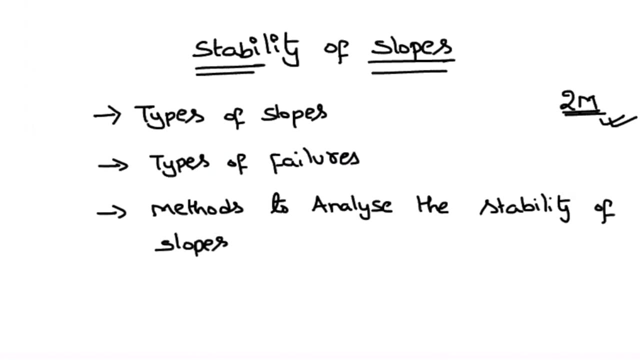 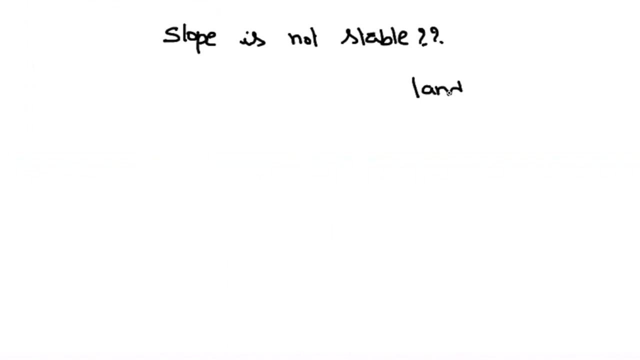 to analyze the stability of slope. So let us first understand what if soil mass is not stable? Otherwise, what if slope is not stable? Then what will happen? then landslides will occur. so if landslides will occur, that means there might be a 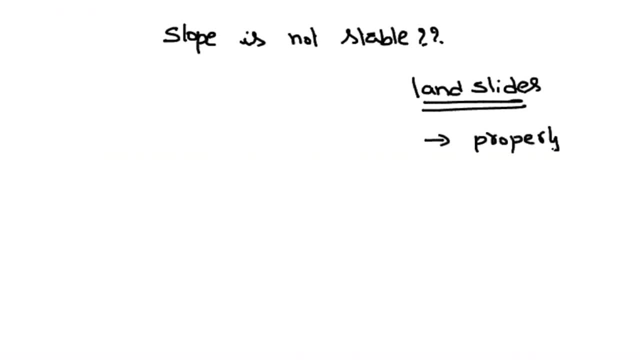 loss in the property and also there might be a loss in the human life, right. so to avoid that, we have to make sure that whatever the slope, whether it is existing or else we are going to make, that has to be stable, to avoid the property of the life and also to avoid the loss in the human life. so let us 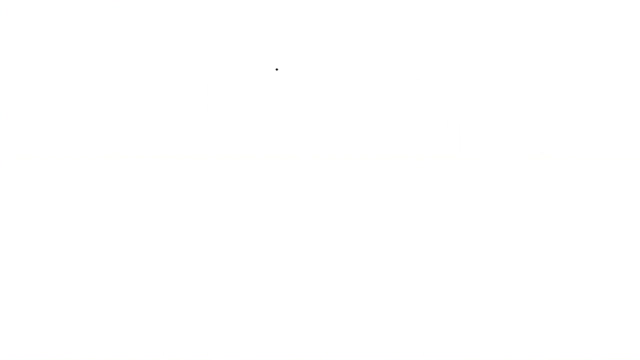 first understand what are the types of slopes. so there are two types of slopes. one is nothing but a infinite slope and another one is finite slope. this infinite slope- normally it is classified as a slope that extends to over a long distance with uniform soil conditions at any depth below the surface. that means if a 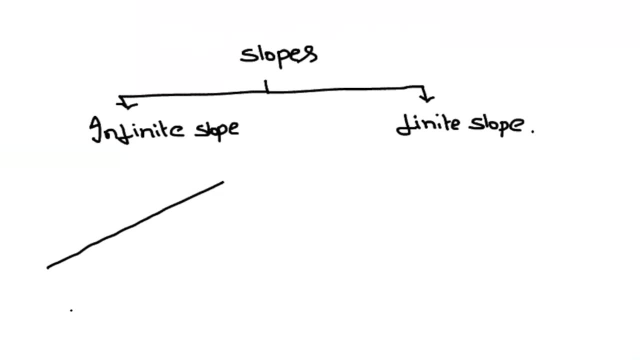 consider any slope, if it is extends to very long distance, then that comes under the infinite slope. and if we consider any layer, if we consider any layer at a certain depth, let us say, if i am considering a layer at a depth h below the ground surface, along the layer throughout the slope, 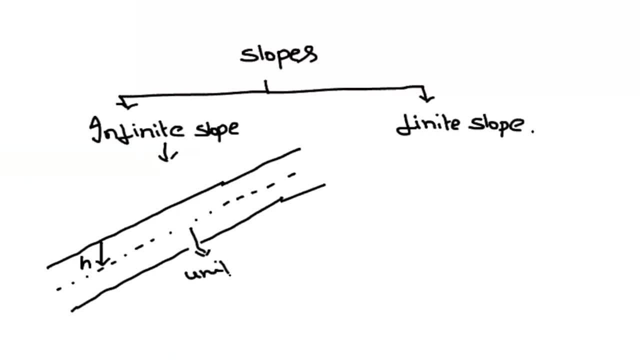 the uniform conditions will exist. remember one point here: the uniform conditions will exist at a particular depth, along the length of the slope. okay, it is not mandatory that these uniform conditions will exist along the depth. also, it may or it may not be so if it is the infinite slope that extends to a long distance. 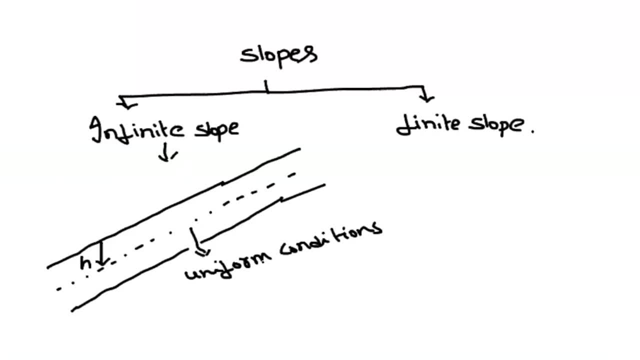 and at a particular depth, we will have the uniform conditions. that means, if i consider, if this is my infinite slope, then it can be considered as a uniform condition. the uniform conditions will be made up of the two different soils. let us say this is made up of soil 1. 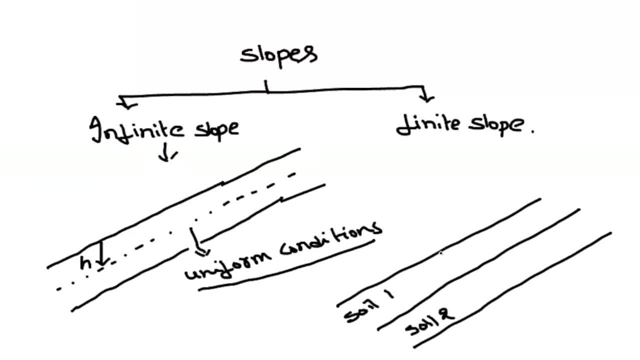 and this is the made up of soil 2. if you see, here, let us say, the soil 1 is up to a depth h1 and soil 2 is up to a depth h2. so the properties of the soil 1 is different and also properties. 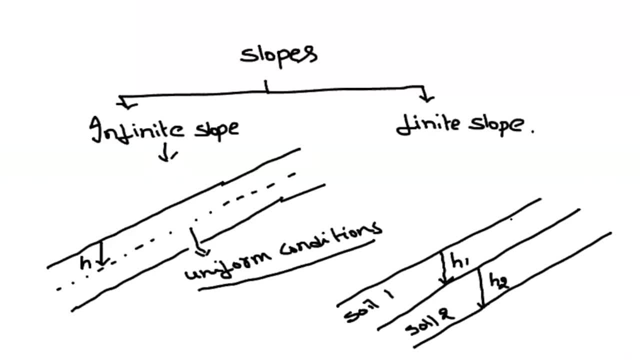 of the soil 1, 2 is different. but if you are going to take at a certain depth, called h, along the depth, the properties are the conditions of the soil will be same. then it will be called as a infinite slope. so what are the examples we'll see under the infinite slope? 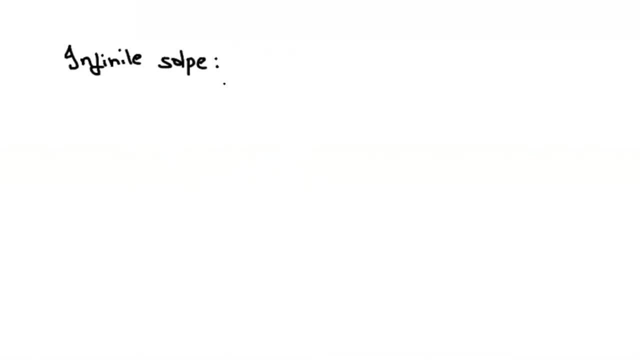 so in most of the cases these are the naturally made slopes, like we can say, mountainous slopes or as we can call it as a hillysides. so these are the best examples for the infinite slopes. now let us talk about the finite slope. so what does mean by a finite slope? or else it is also called as a man-made slope. 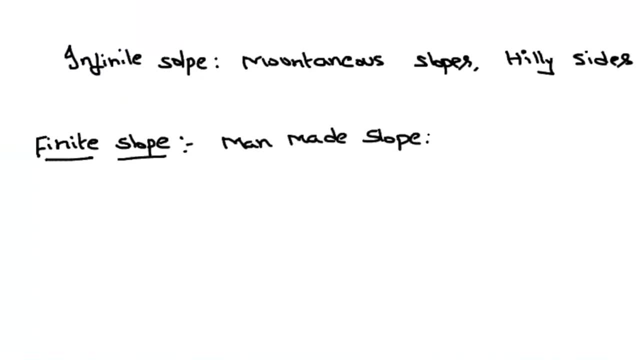 why we have to make the slopes. suppose, let us say i am having land at one level and if i want to connect this land to the and i cannot connect it to the other land, land to the another level, then we have to make a slope here. so why we have to make a slope? so 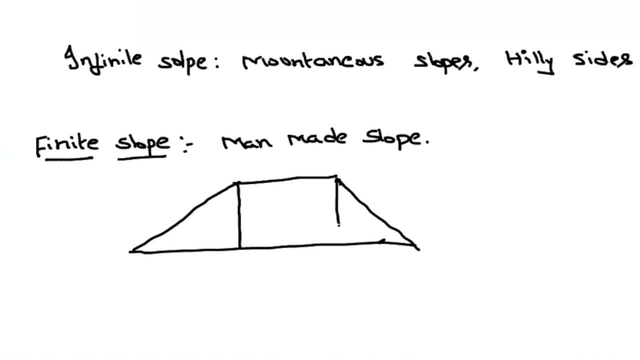 why can't we just simply form a soil with this shape? so what will happen? the soil cannot itself retain itself along the vertical direction, so that's why we have to- for the stability we have to make certain slope to connect to the another level. so what are the examples for this? 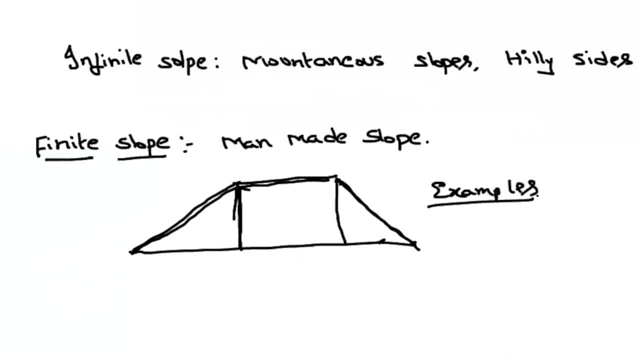 what are the examples we'll see? suppose, if you're going into the road embankments- i think everyone must have seen it- whether in road embankments, or else we can see in rail embankments. we have to maintain some level, to maintain the some characteristics, whether it may be a highway. 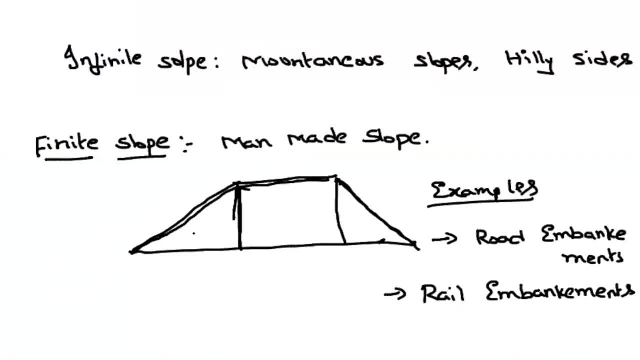 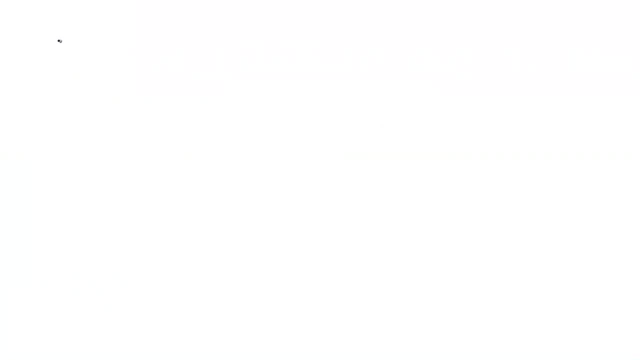 or it may be a railroad. so that's why what will happen? we have to change the levels from one point to another level. so in that case we will use the, or we will construct some slopey surfaces, or else that we call it as a embankments, or else what are the? any other examples? suppose, if you are 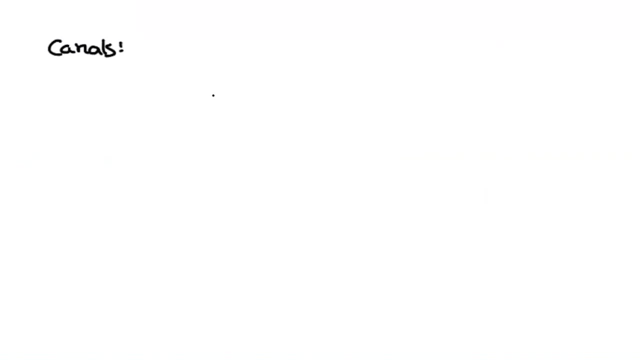 constructing some canals and canals. what will happen? again? we will have to maintain some level. we will make some embankments like this and water will flow in this slope. so again, here also we have to make sure that the slopes of the embankments must be stable. so in other examples and also we 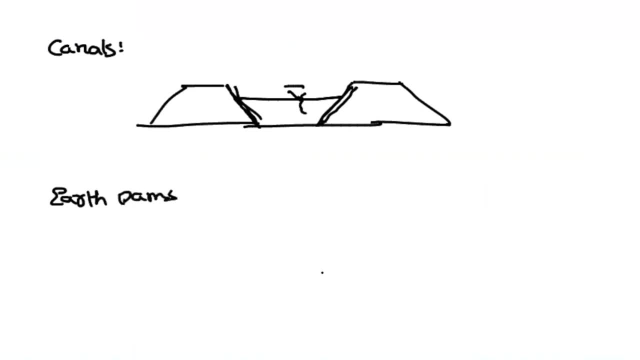 can see earth dams also. if you want to retain level on the very or if you want to divert the level water, then we can, in world and as they are used to construct the earthen dams if you want a, if you want to retain water at the very high levels. so in this case also,